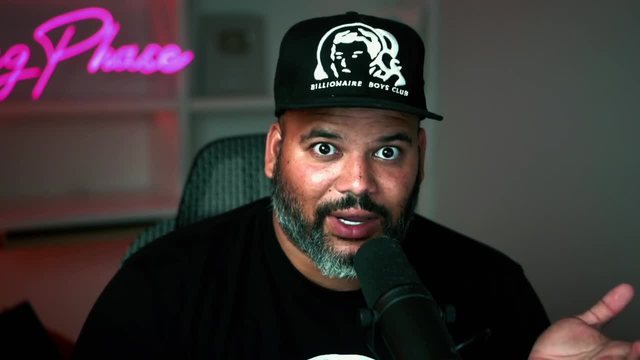 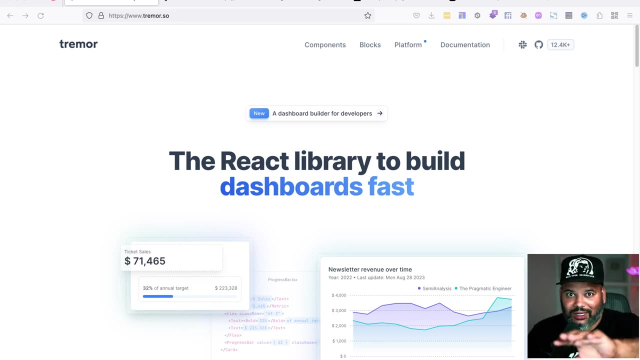 then this is some of the best resources that I'm about to give you right now. Okay, so let's get into it. All right, guys? you already know it's your boy, Joe. back at it again, CodingFacecom. If you like this type of videos, make sure you subscribe and you like the content and leave a. 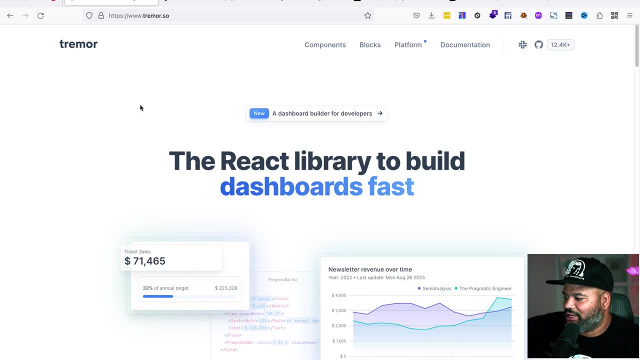 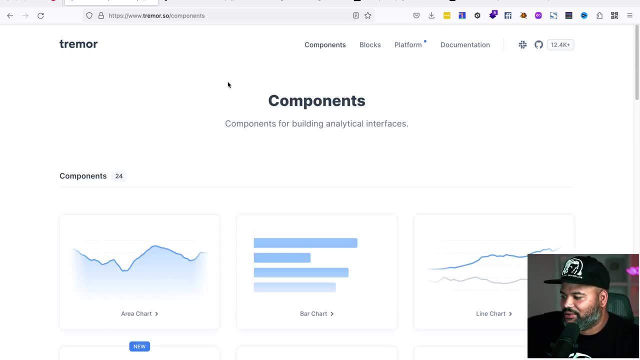 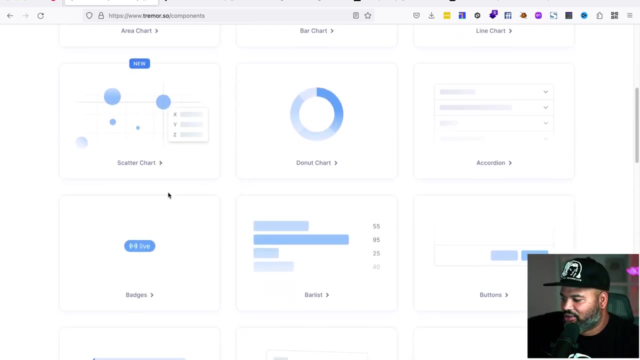 comment. Tell me what you think. Okay, so today I want to introduce you guys to Tremorso. So this, right, here is a React library. right, to build dashboards fast. Okay, it's a series of components. right, You have things like area chart, bar charts, line charts, scatter charts, donuts. 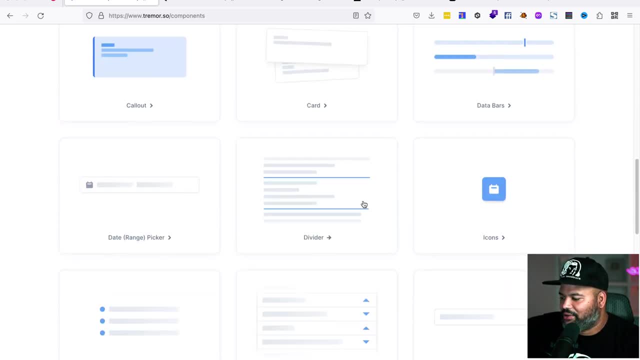 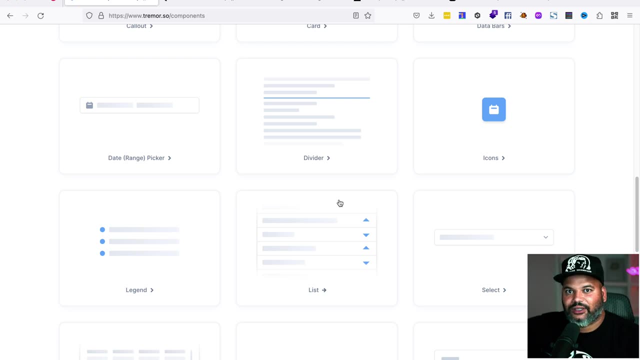 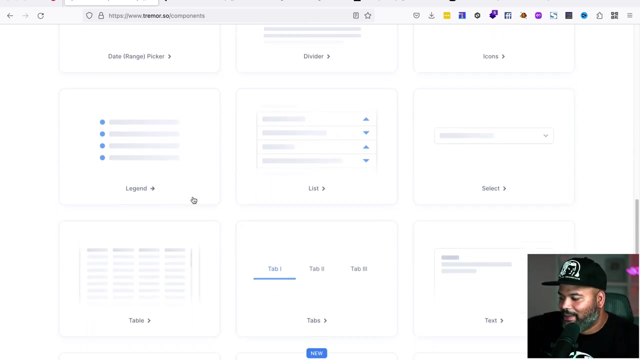 right accordions. Again, pretty much everything that you need to start building a dashboard Now. again, this is really useful for someone building some type of full stack application and you want to have an admin section or a dashboard for the user to see some data and some stats. Okay, instead of 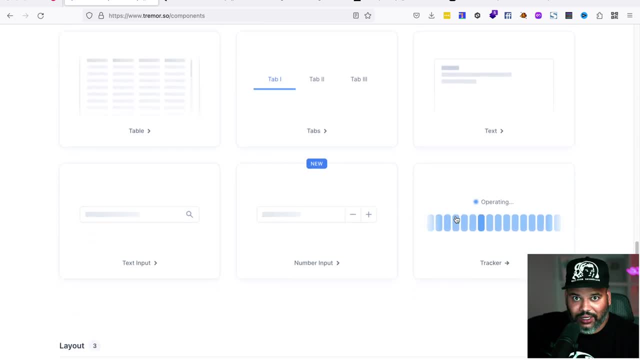 you having to build everything from scratch. come in and use this library And again all of these libraries that I'm about to show you guys right now. they're pretty much free, So they're open source, So any one of you guys can use it without having to pay a dime, which is always a good thing. 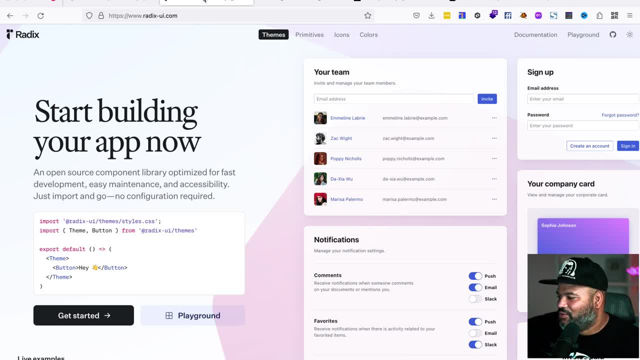 right Now. the next one that we have right here is called radix-uicom, And I really like this one because it's very nice and clean. There's a lot of different examples of things that you can use, So again, you could theme this out, right, You got? 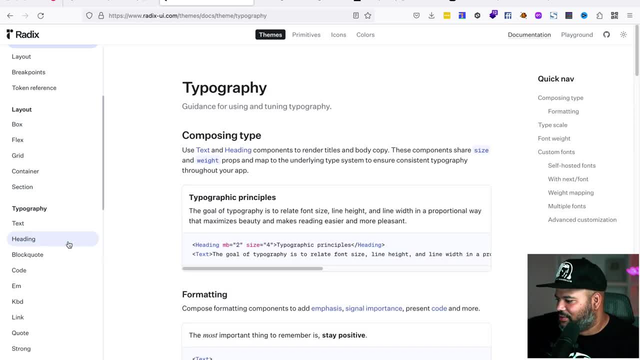 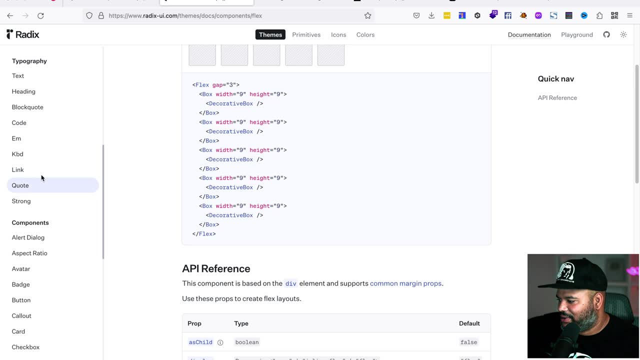 colors right. Dark mode right- Typography- that's already laid out for you. You got things for your layouts right. You have grids flex right. Again, it's just to make your life much easier. You have things like a container right- Let's get into it. So let's get into it. 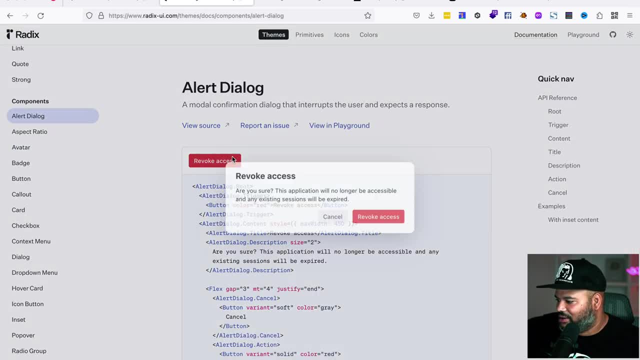 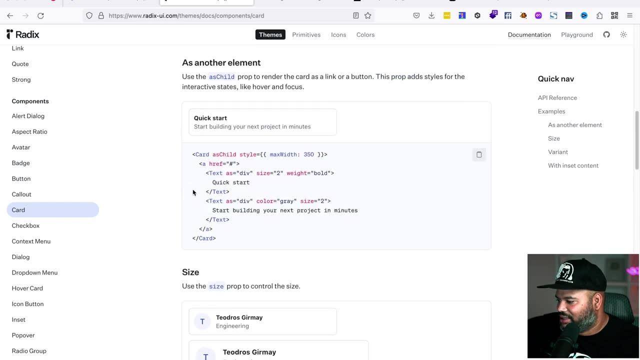 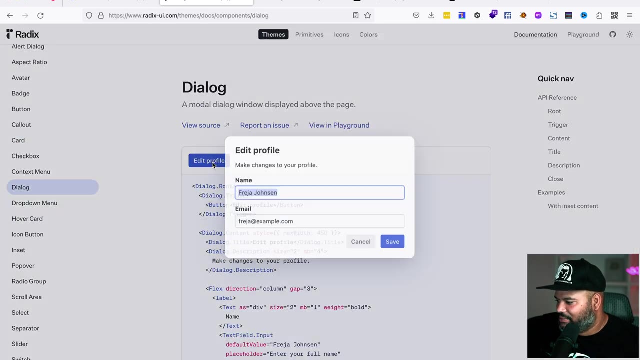 So let's get into some of the components that it has. You have an alert right Again, aspect ratio badges, avatar cards. Again, you have different examples of things that you can go and build. So it's really to save you some time, As you can see edit profile, which is like a dialogue. 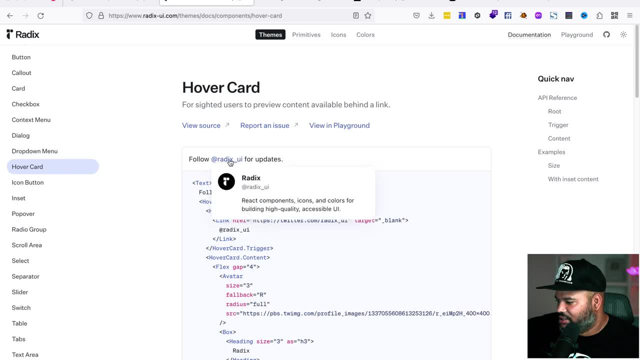 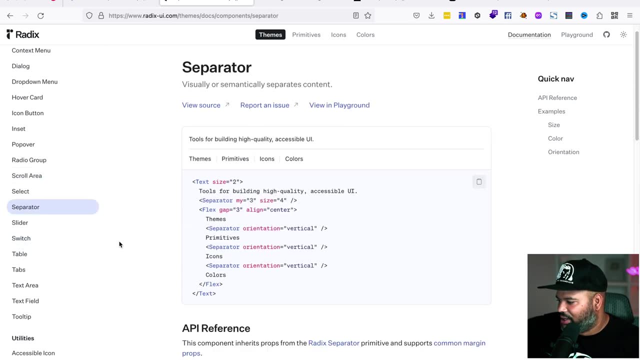 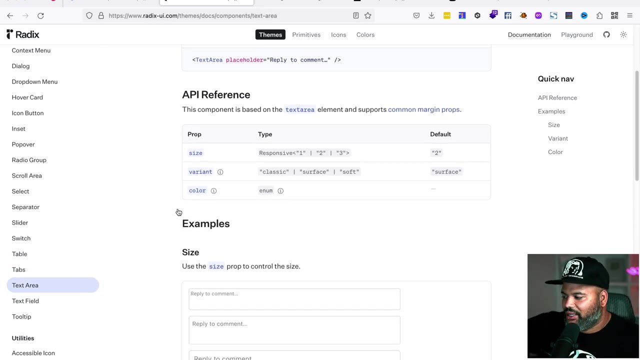 right. You have other things like hover cards, As you can see here. you have insets, scroll area separator. You also have tables, tabs, text area, So pretty much everything that you need to start building a web application And again, it has a lot of utilities that you 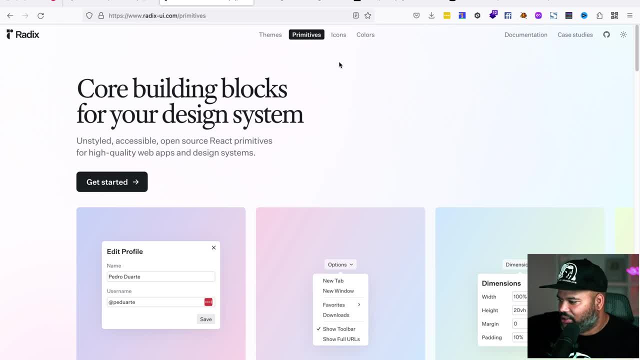 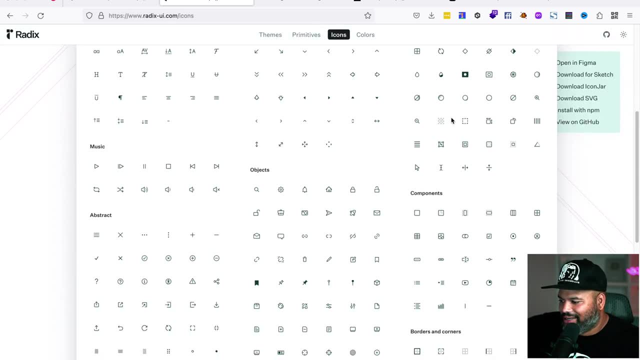 can also use Another thing that's pretty cool. it has some primitives right, Some examples of things that you can build with it. You also have icons. Again, if you're looking for some really clean icons, this is one of the best ones that I've seen. Another thing that you can do is you can 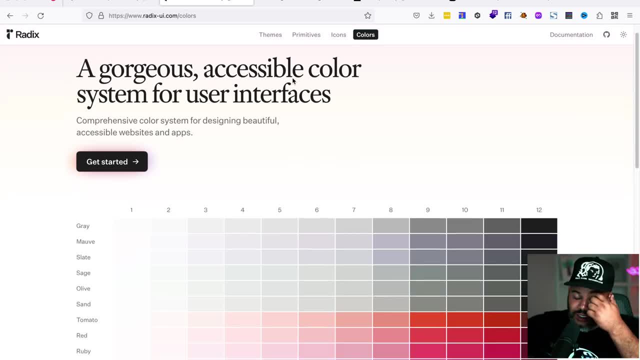 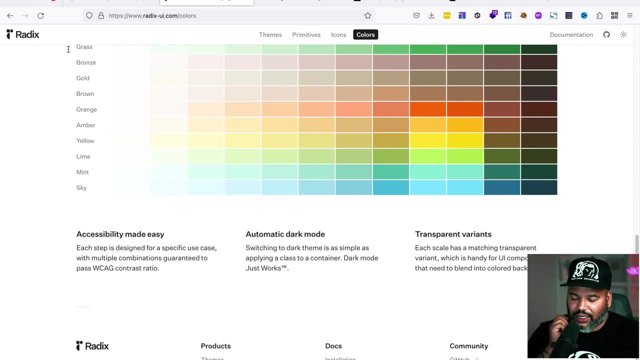 have a web application. So if you want to do a web application, you can have a web application. So if you have again is colors and you know accessible colors, that can really work in a situation okay. so that's radix. right there, guys. now again guys, if you want to learn how to code and you- 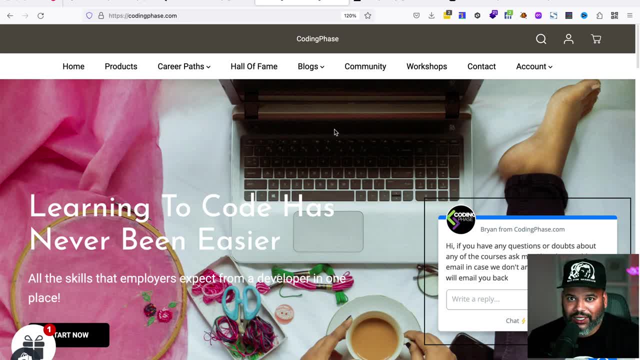 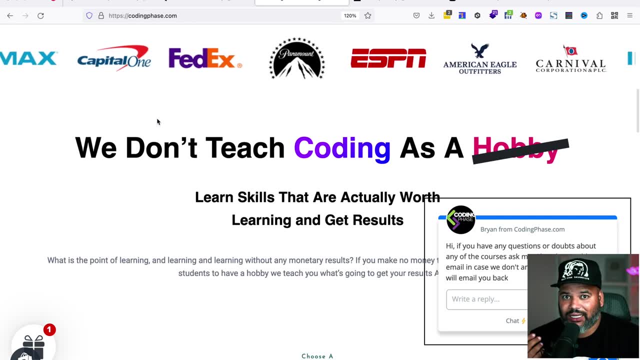 like this type of content. trust me, you definitely want to come to codingphasecom and try the service out. pretty much we don't teach coding as a hobby. we focus on the things that's going to get you a job or you can start freelancing with or start building your own business, if this is. 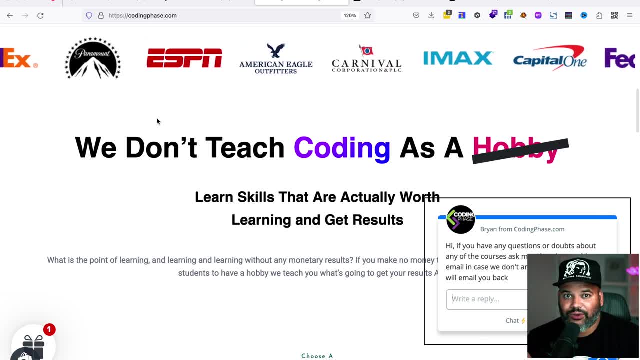 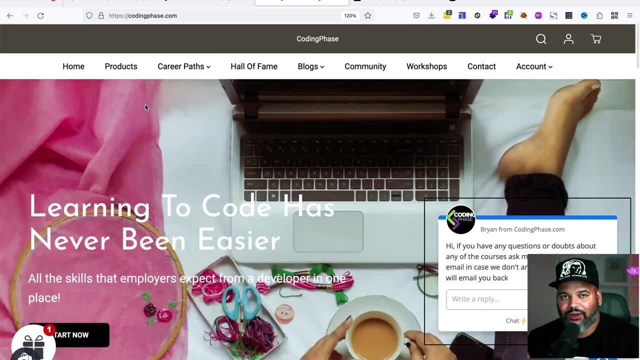 something that you're really passionate about and you want to start doing. guess what? definitely come to codingphasecom. we have the gold membership, diamond membership, right, uh? so anyone with any type of budget can come in and get started. now again, you can always come in, check out the hall. 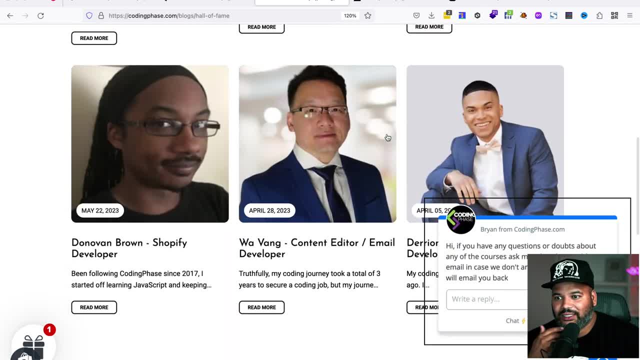 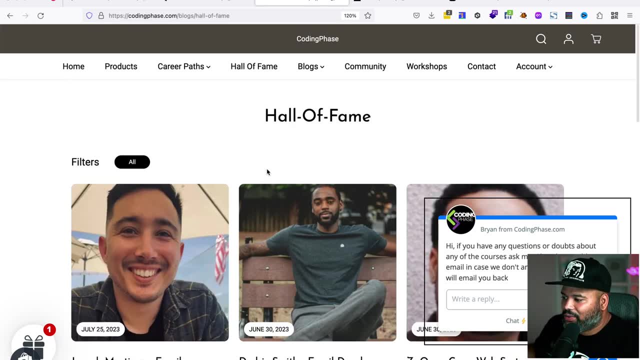 of fame. right, don't believe me. check out some of the students that we've had success with and people that have, uh, came through coding phase and are killing it right now. okay, so yeah, let's go to the next one that we have here now. this one is a very popular one. 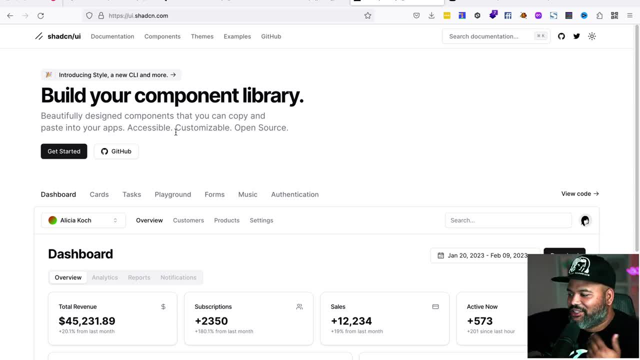 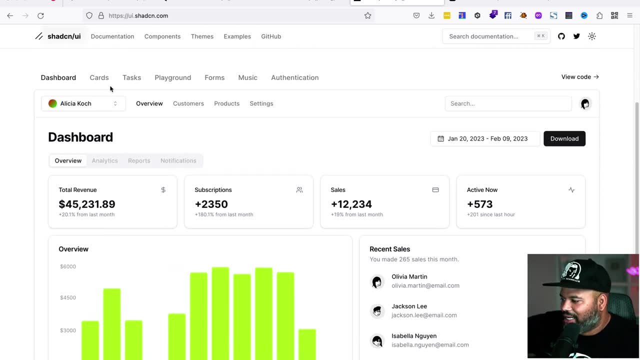 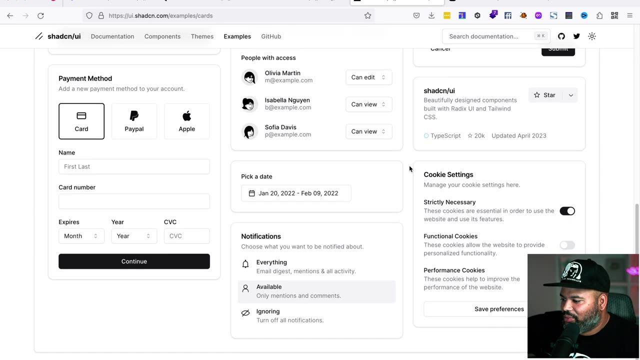 which is chat dcn, not chat cdn, but chat dcn, um. again, this one's another one that you can use for dashboards. right, they have a lot of different examples of things that you can do with their components. you have different cards. again, if you want to build like a ui for some type of 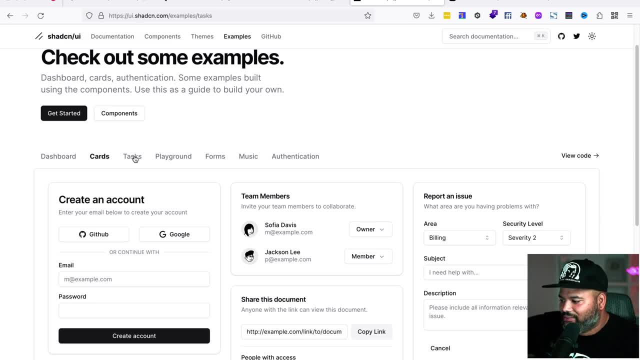 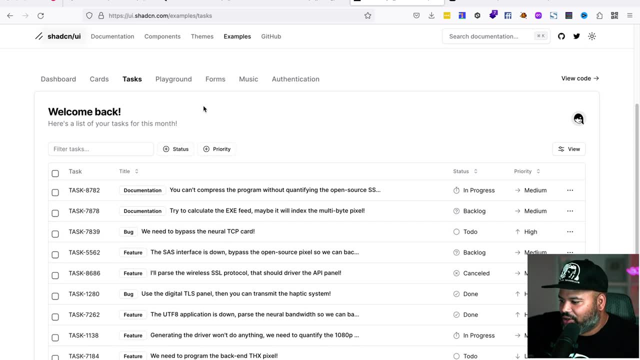 application that you're building, especially with full stack. this pretty much gives you every simple uh example that's out there for you to use, and i'm going to show you how to do that in just a second now. once you've built this, that's it's done, so let's go to your github and see how to go. 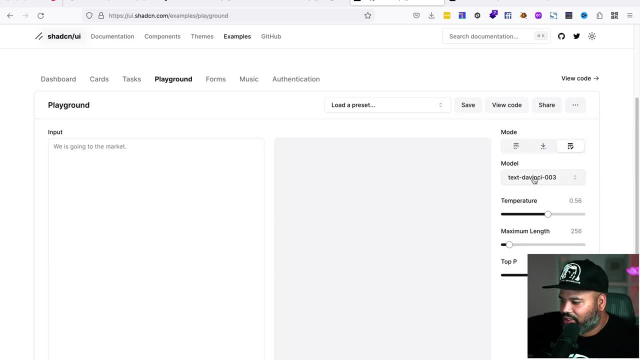 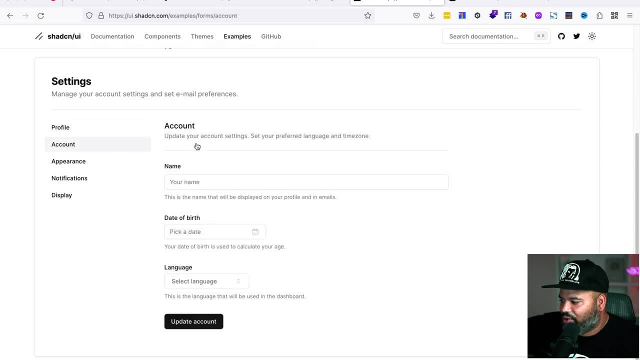 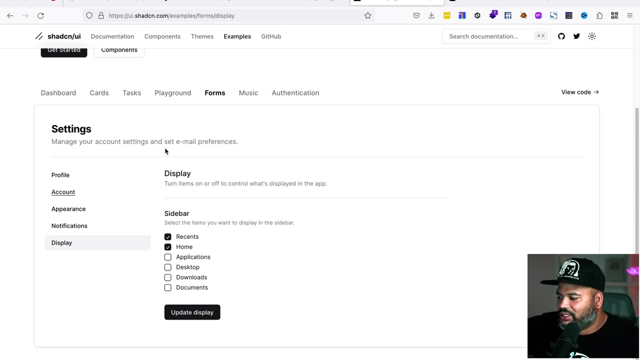 with it. you've got different modes, texts, right, um, you also have forms, so you can see here some examples how, let's say, a profile page could look like: okay, now again, you could go in and style this however you want. but what's really cool is that the components are there already pre-built for. 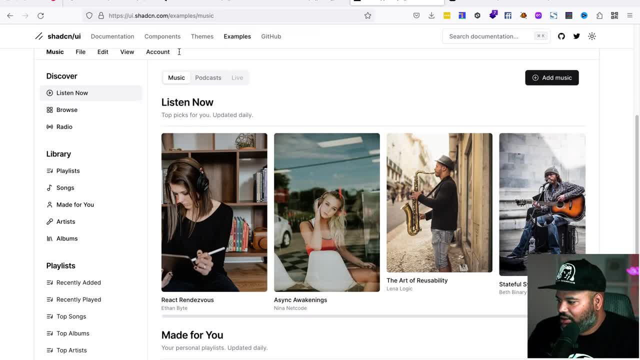 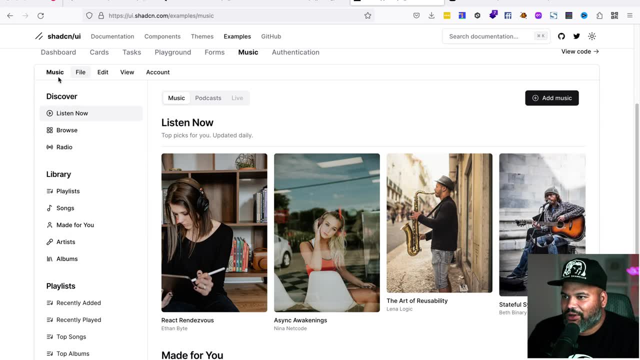 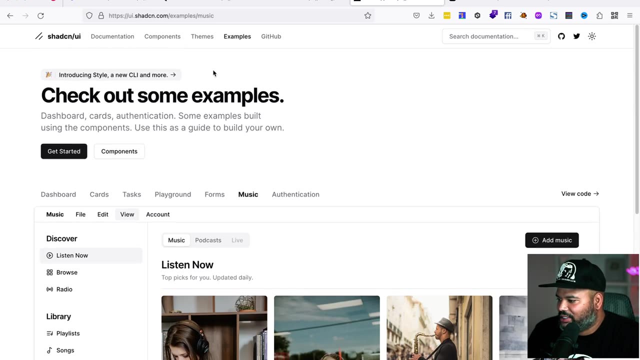 you, so definitely pretty cool. again, you have some examples here. if you wanted to create, like, some application for maybe electron, as you can see, you can even have your, your top menu already set up for you. again, it's a lot of different things that you can do with this and, yeah, man, you can see all. 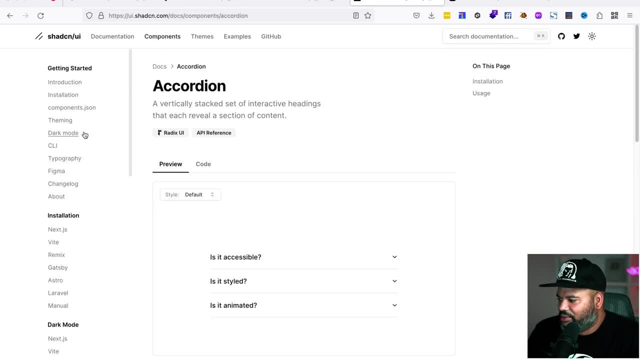 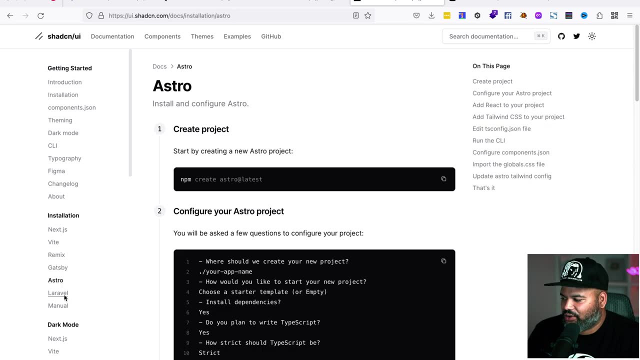 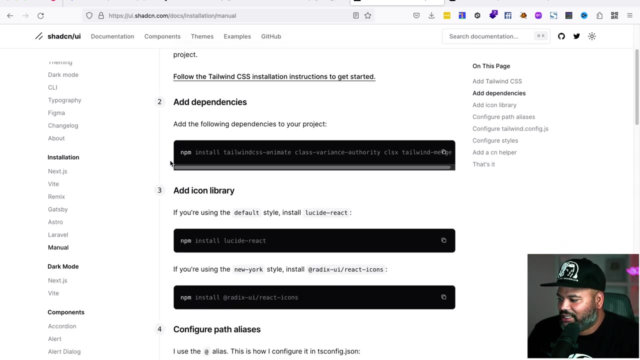 of the different components, and what's really cool is that you can pretty much integrate this with anything, especially like nextjs, veet, remix, gatsby, astro, laravel and just manually for any type of project that you might want. again, this does add tailwind css, so if you're using tailwind, 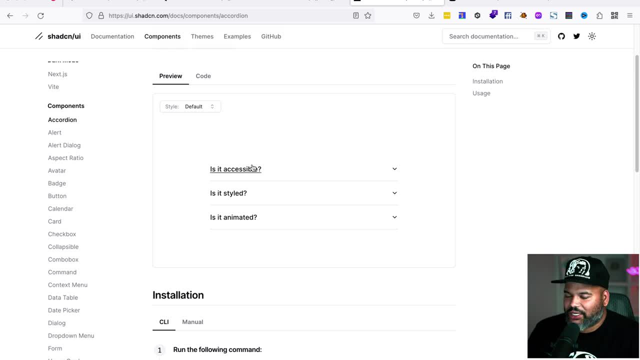 this is going to be something that you can use and pretty much get started now. for those of you guys that don't know, tailwind css is just pretty much utility classes, so it's pretty bare bones right. so i know somebody that's coming from bootstrap. they might say, well, why would i use? 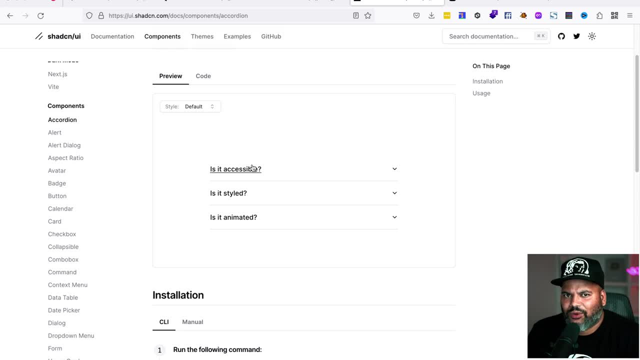 tailwind, when you know none of the components really work or you know are actually something that i can use um on day one, right away, And it's like I have to write the JavaScript. Well, guess what? This is why you use one of those components libraries where they're using Tailwind CSS and you can 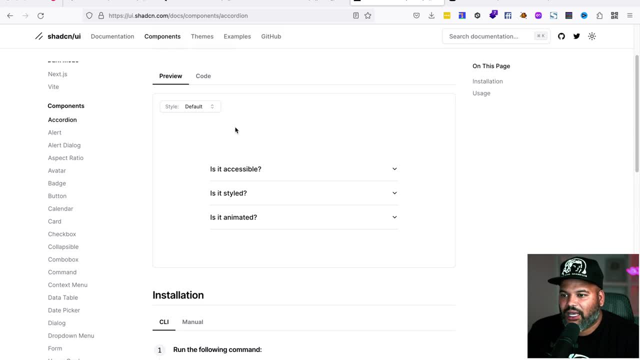 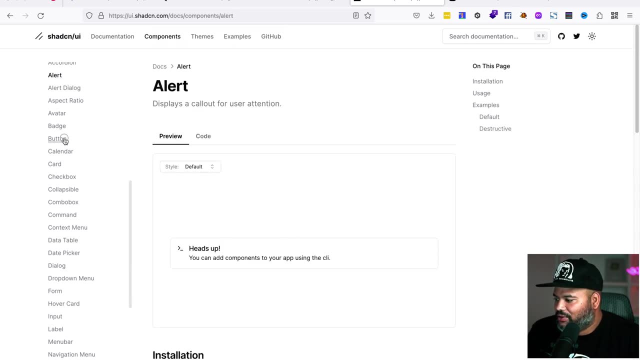 still customize it however you want using Tailwind, But at the same time, you already have all of these components here that work for you perfectly. Again, you have buttons, you have commands right. You have date picker right. If you guys have seen this, this is one of 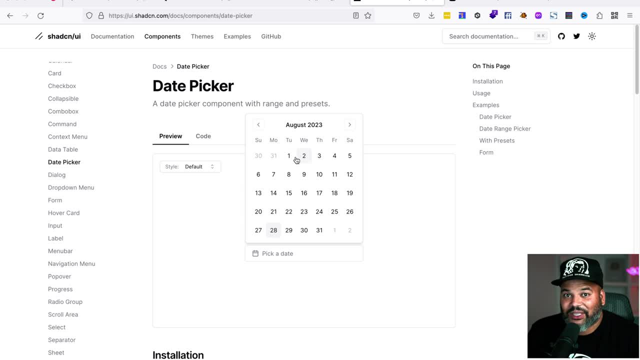 the most difficult projects that you can do as a beginner. you know building with JavaScript right. A date picker is not as easy as people might think, So guess what? You could go in and choose something like this, where it's already prebuilt and all you have to do is style it. 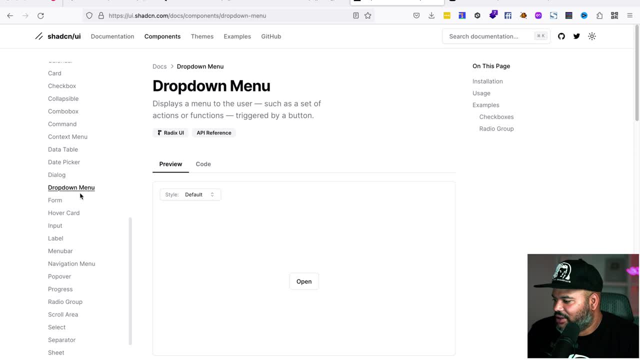 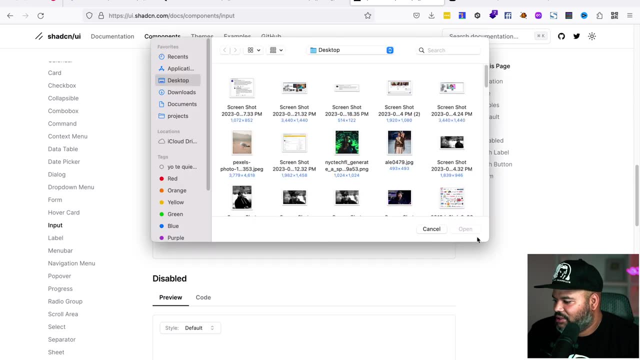 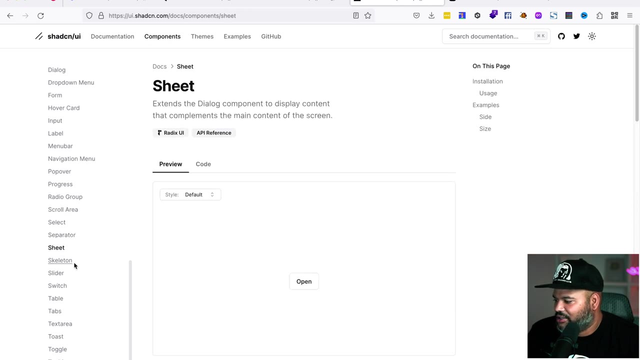 however you want. Okay, So again you have drop menus. you have input fields- right. Different examples of input fields that you can use. Okay, Let me see what else we have in here. Scroll area you have selects separators right. Sheets skeleton- right. When the data is loading up, you can use. 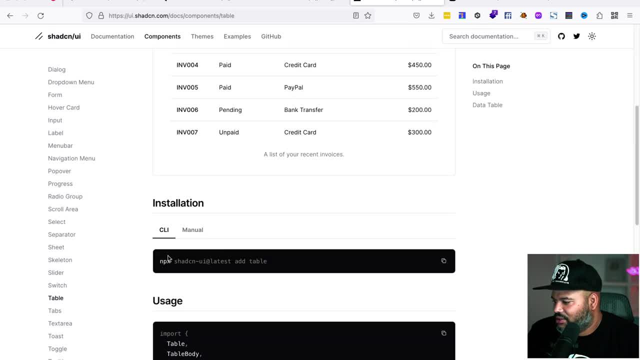 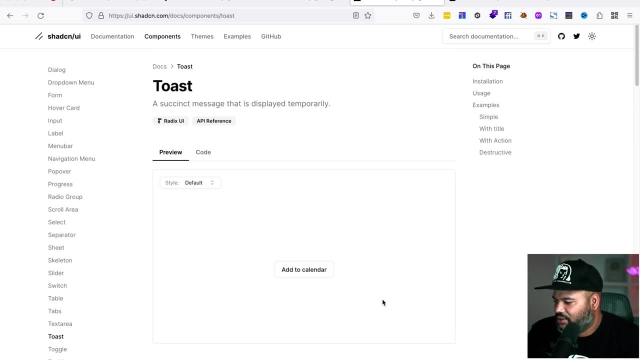 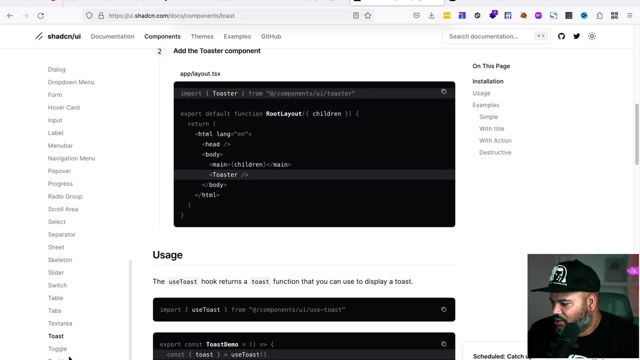 that. Again, you have tables, of course. So text area toast. Okay, You see, like the little menu or the pop-up modal that pops up at the bottom, Okay, So you can use that. So yeah, this is pretty cool. Again, this is called ShadCN. You can definitely check it out Again. I'm going to 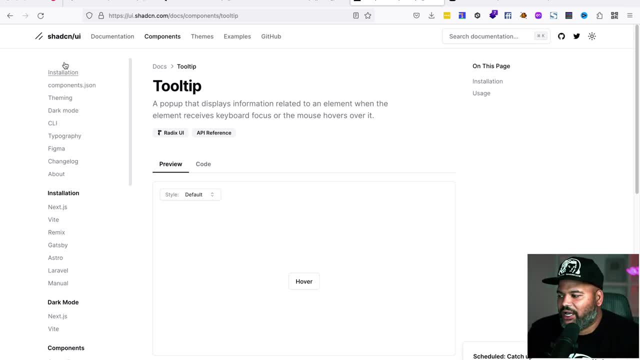 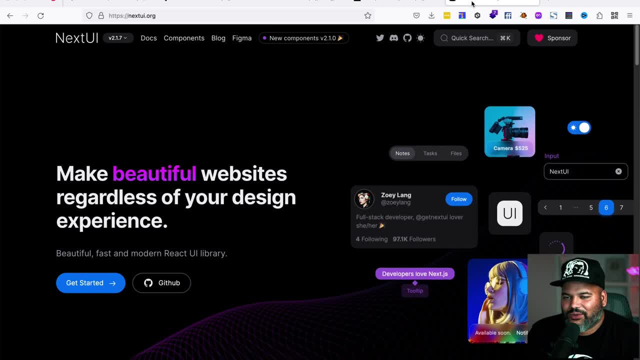 on your own time, Then the last one that I have here is one that, to me, is probably like the most beautiful one, especially when you're somebody who might not have like a background in design and you just want to start building something that looks really good, But again you want to. 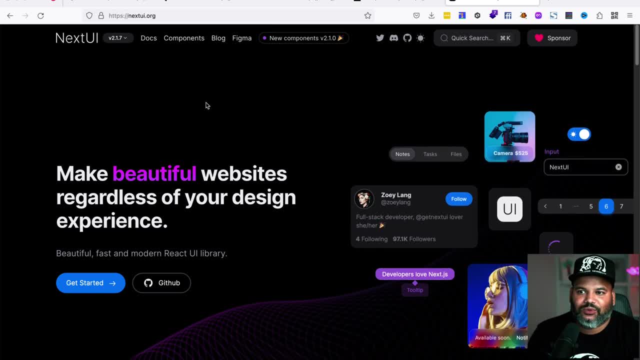 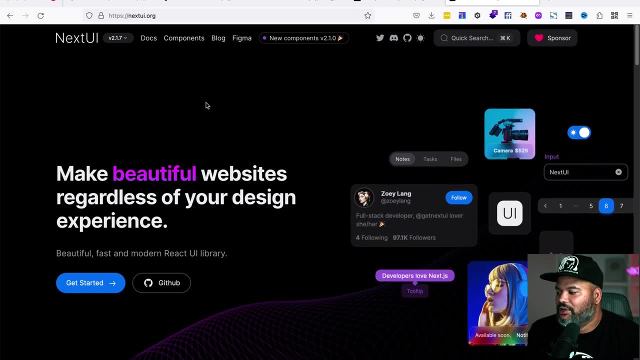 focus on the functionality of your application. You're like: okay, what do I do now? Do I have to now become a designer? No, guess what? You use one of those libraries and you're like: okay, to help you build beautiful UIs and get you started Again if you go over here. 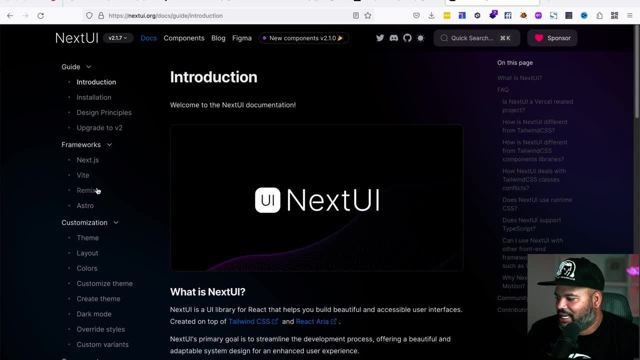 you have the documentation. This pretty much works with everything that's out there: Nextjs, VEEDS, Remix, Astro. Again, these are React components, So you're not just stuck with doing it with like the JavaScript way, like Nextjs and, let's say, Remix, You can also go in. 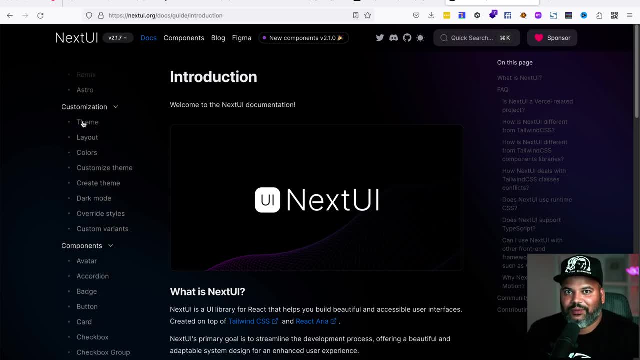 and use those components for an application that you're doing with, maybe Laravel or maybe C, Sharpnet, right Or Java, et cetera. You can pretty much use this and start building some pretty cool websites. So, as you can see here, this is like avatars that you can use. 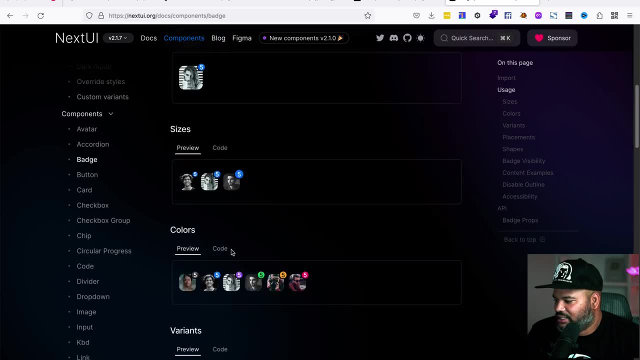 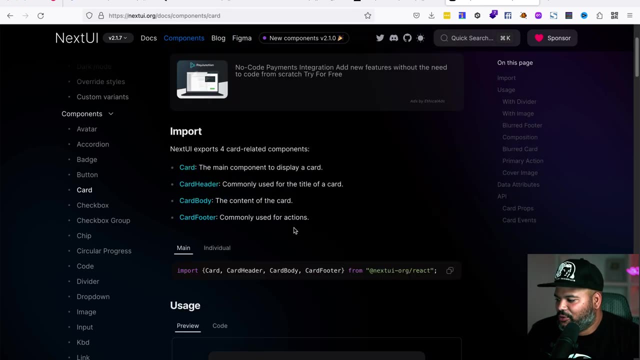 You have badges, as you can see, right. So again, there's a lot of little things that you know, just save you time, that you might need for your application. but you might say: you know what, Let me see if I could get a designer for this. Let me see if I 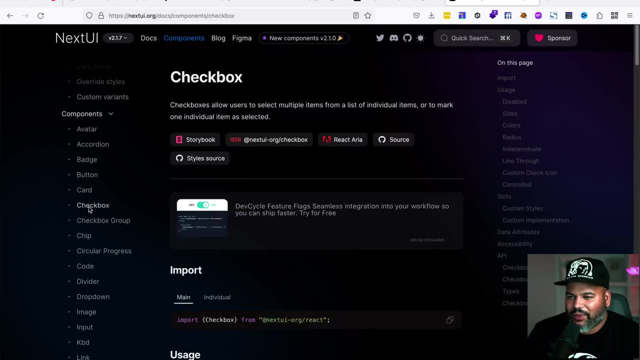 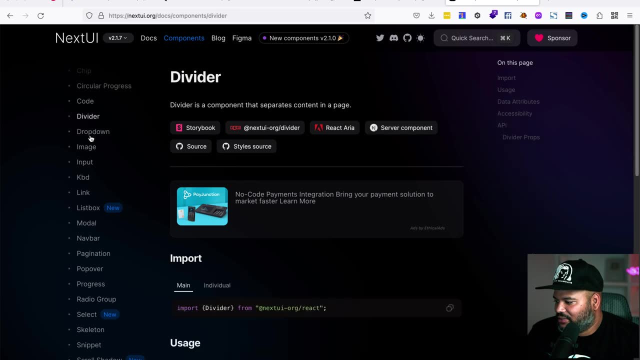 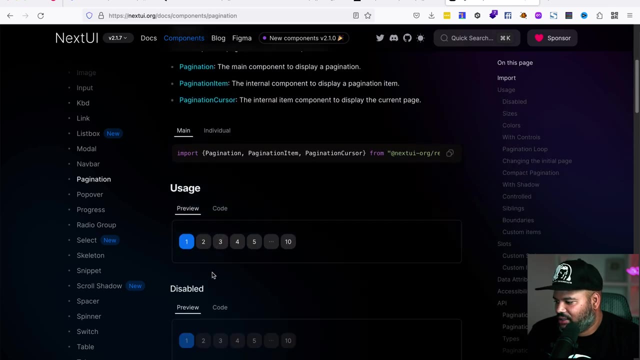 could go get somebody else to build this for me And it's like, okay, you might as well just use one as a library and just save you that time, Okay, So again you have dropdowns, dividers, images, So as you can see pagination right, And it looks really good Like I'm not going to lie. 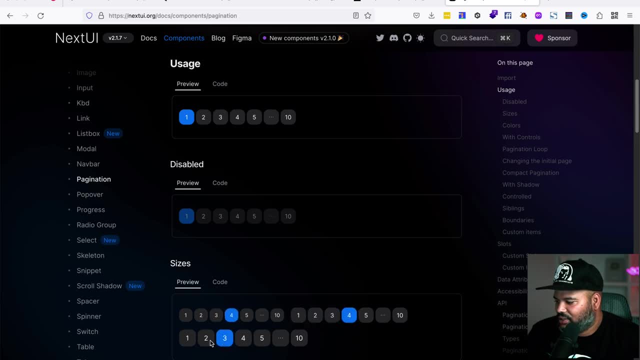 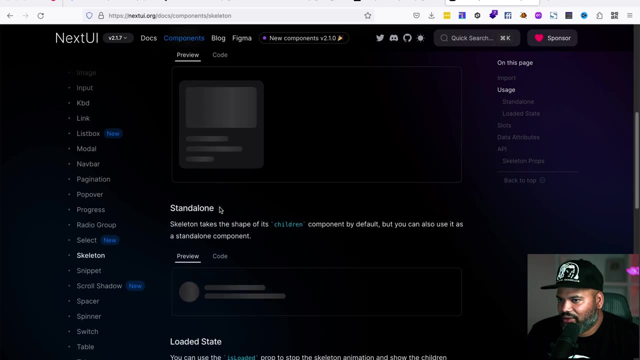 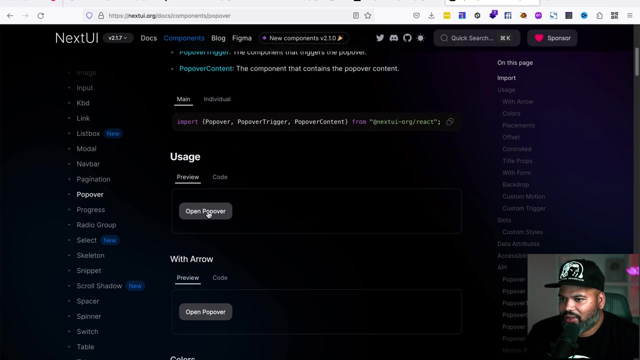 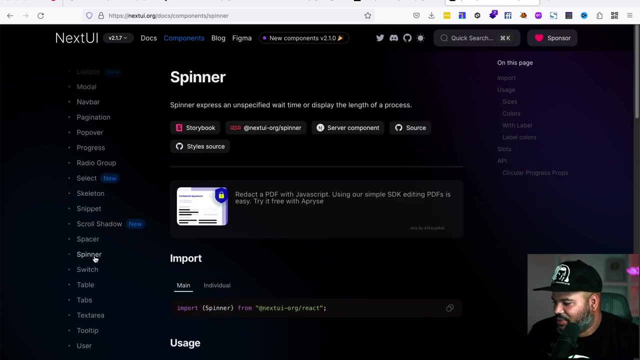 like this is really nice, very smooth. Okay. Again, you have skeletons over here, different examples Of how you can use it when the data is loading. All right, You have the popovers. Okay, As you can see, you have your scroll shadow. You also have like a spinner, If you might need one. 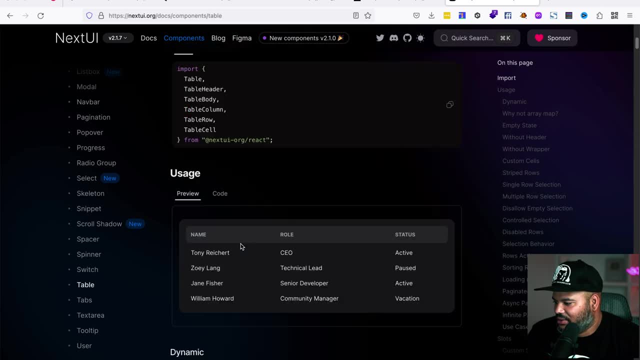 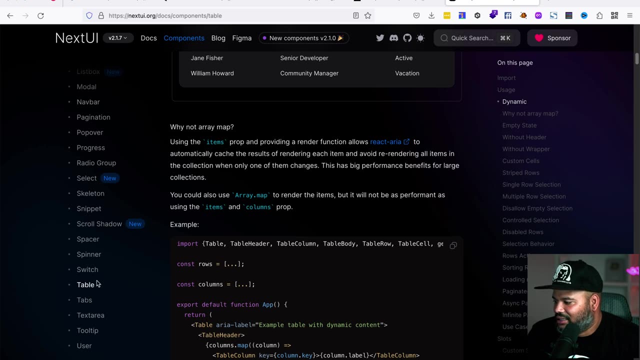 for your application. you have different tables, Okay Organized And, as you can see, this was, it has like more of a design and like a design style for this. but, um, all the other ones you can customize and just like this one. you can customize it as much as. 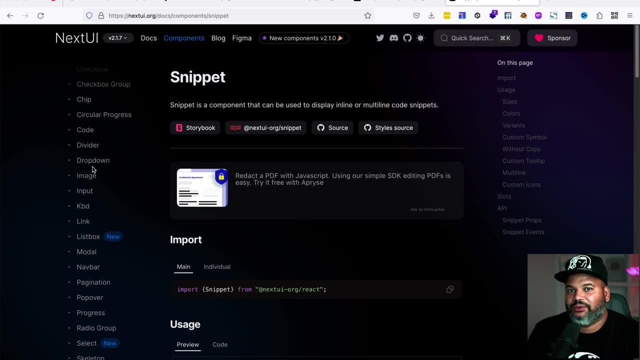 you like: Uh, you're just using the components to be able to speed up your process of building the application, So you don't have to do everything from scratch. Okay, So definitely go check it out, guys. Um, again, I want to give you guys some quick videos, just like this one where I just 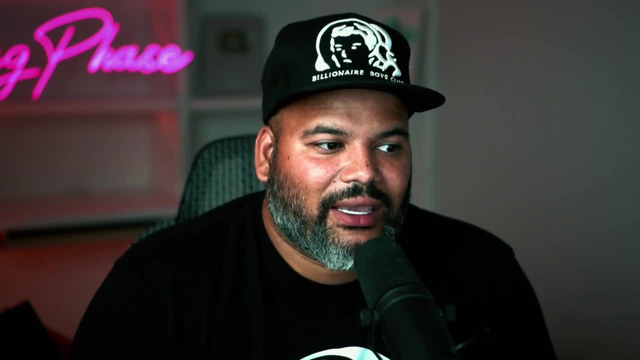 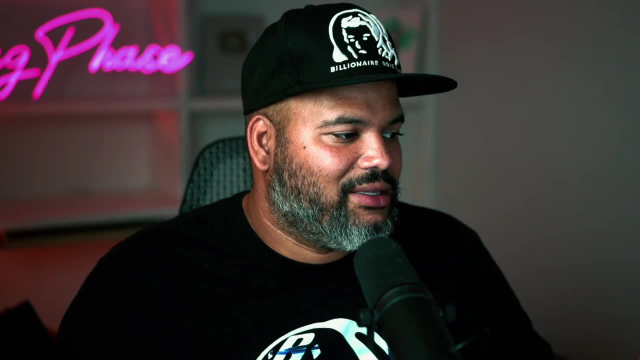 come in and give you guys some resources, as I find them. And, yeah, man, definitely go subscribe to the channel. Show some love, Tell me what you think. which one have you ever used from this one? Chad DCN. Have you ever used um tremor? Have you ever used something like the?